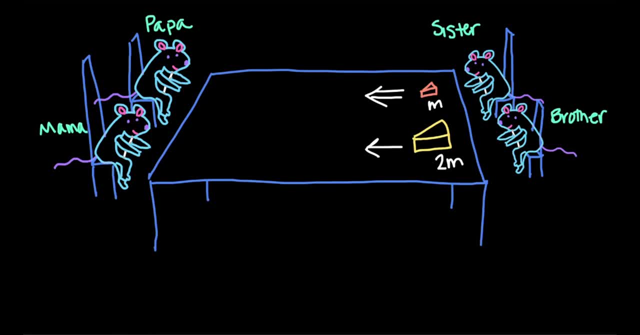 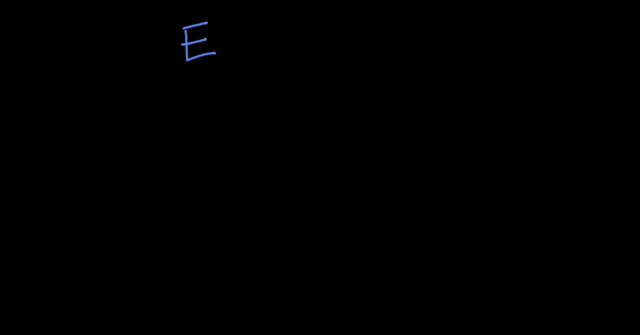 cheese has more kinetic energy. In fact, it turns out that it's the swiss. in this scenario, Kinetic energy depends on both mass and speed, but the dependence on speed is stronger. This estimation of kinetic energy can be quantified in an equation that lets us: 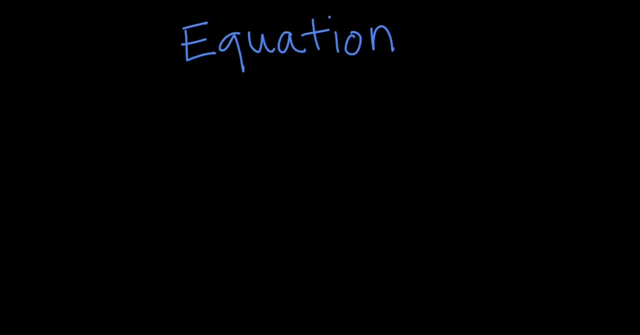 calculate kinetic energy exactly? We said kinetic energy depends on the mass and the speed, which we'll write as v for velocity. so we can start with: ke equals m times v. But we said that it depends more on the speed, so the velocity here is actually: 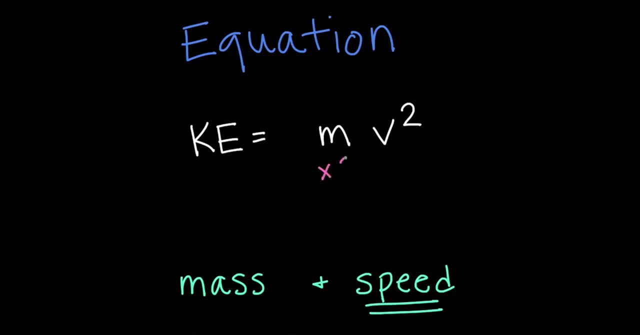 squared. This means that if an object's mass doubles, its kinetic energy also doubles. But if its speed doubles, the kinetic energy actually quadruples. And there's also a kind of constant factor of one half at the beginning of the equation, but we won't go into the details. 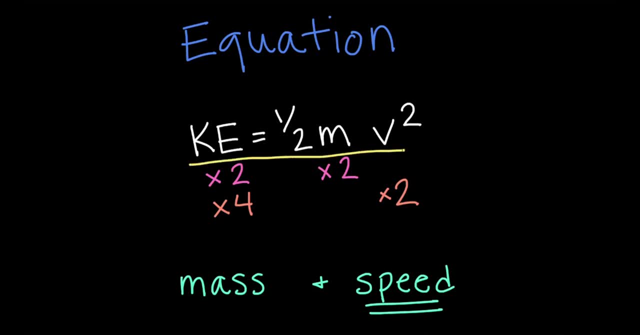 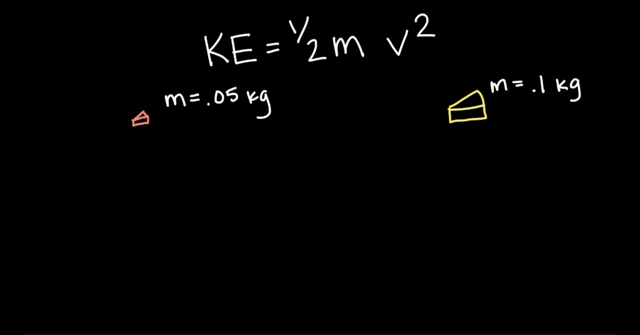 of the math of deriving this today. So this is the equation for kinetic energy: one half mv squared. Let's apply this equation to our cheesy example. Say the swiss has a mass of 0.05 kilograms, which makes the cheddar's mass 0.1 kilograms, When both cheeses have the same speed. say 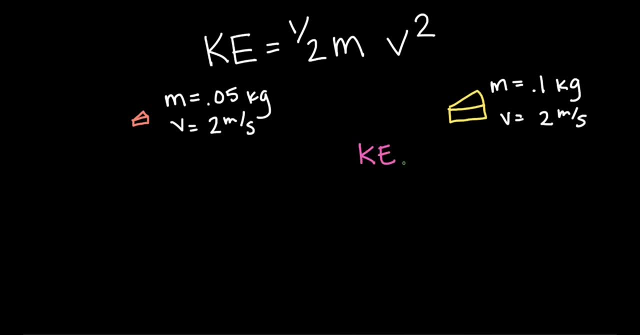 two meters per second. the cheddar's kinetic energy is one half times 0.1 kilograms times two meters per second squared, which is 0.2 joules. The Swiss's kinetic energy is 1 half times 0.05 kilograms times 2 meters per second squared, which is 0.1 joules, or half the. 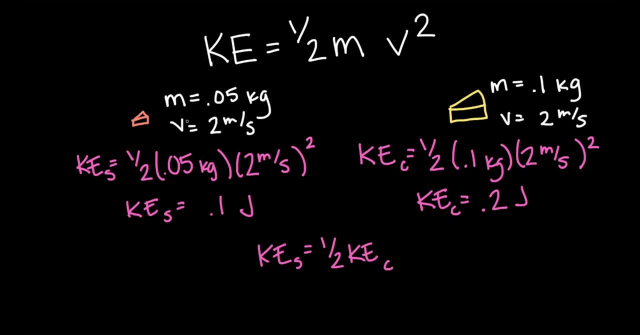 kinetic energy of the cheddar. So we can see that at the same speed the cheddar has more kinetic energy because it has more mass. But when the Swiss has a speed of 4 meters per second and the cheddar still has a speed of 2 meters, 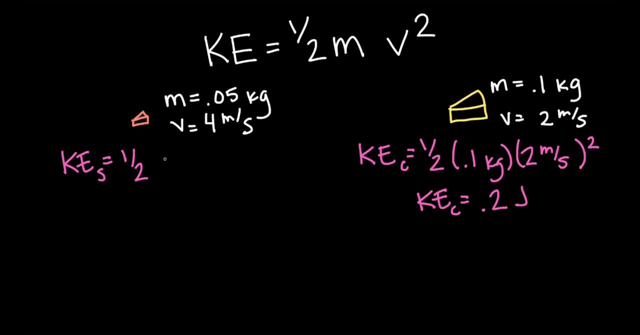 per second. the Swiss's kinetic energy is now 1 half times 0.05 kilograms times 4 meters per second, squared, which is 0.4 joules. So now the kinetic energy of the Swiss is twice the kinetic energy of the cheddar. So we can see that even 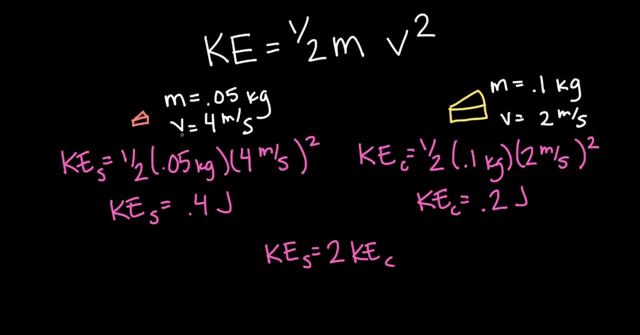 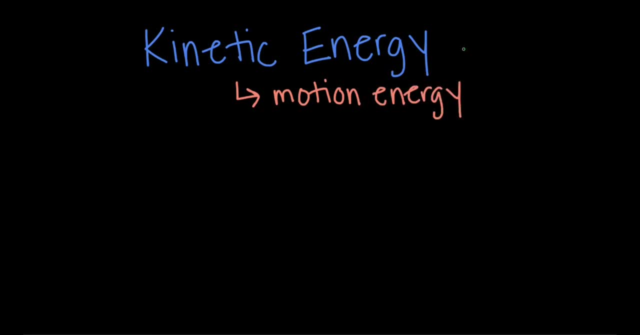 though the cheddar has more mass, the Swiss has more kinetic energy because it's going faster. In summary, kinetic energy is the motion energy of an object. The equation for kinetic energy is one half NV squared. So as mass increases, kinetic energy increases, like the more massive cheddar versus the Swiss.